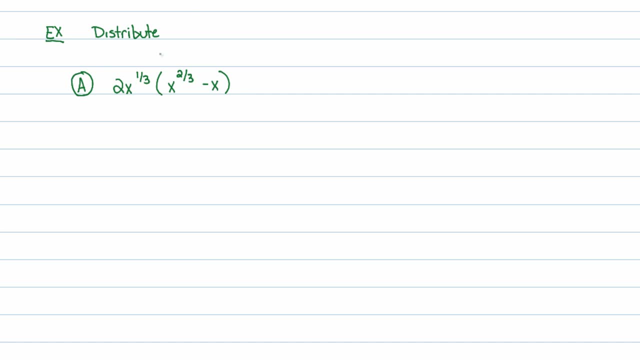 worth its weight should talk about this topic. Distribution here acts like distribution anywhere. You take an object and you distribute it to each of the objects within that expression. So each of the terms there gets a two x to the negative or two x to the one-third attached to. 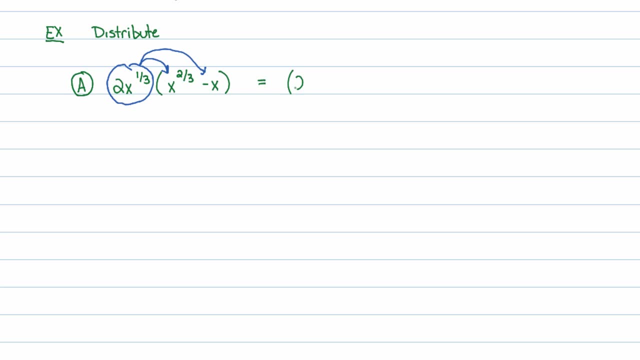 it. So let's see what happens. This is going to be two x to the one-third times x to the two-thirds, Minus two x to the one-third times x, And that's, by the way, x to the first. 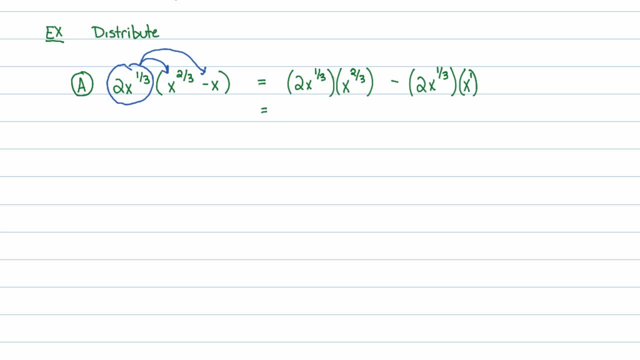 All right, this first product here will have two and it'll be. we're just going to use law of exponents here to add these exponents. That'll be one-third plus two-thirds. The second product will be two times again. since these two bases are the same, I'm just going to add their exponents. 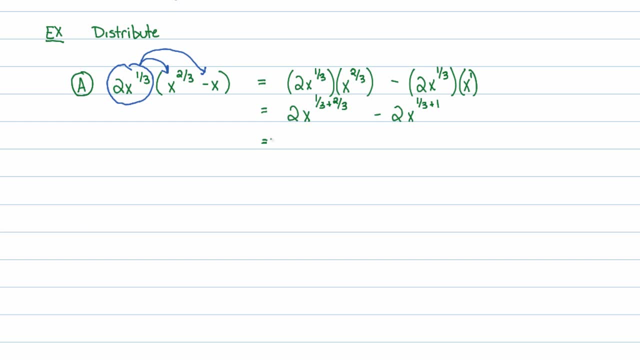 One-third plus one. You should be an expert at adding fractions. at this point. This is two times x to the three-thirds, or first, And this will be two x to the four-thirds once you add those fractions. One last little step here. A lot of people don't like to have ones on their exponents. 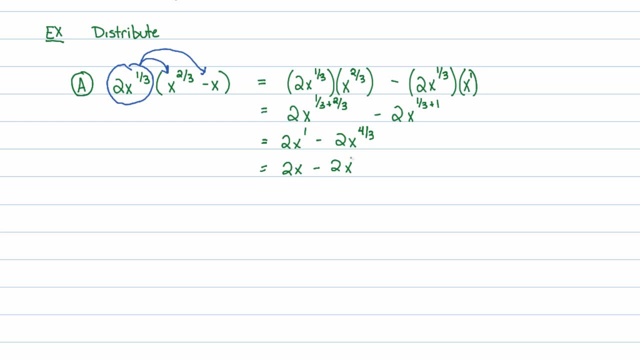 The one is already assumed, so it'll just be two x minus two x to the four-thirds power. That's it. That's it for that one. The idea of distribution is that you're essentially creating more terms than you originally had. Originally we had- and maybe I should make this more apparent by erasing- 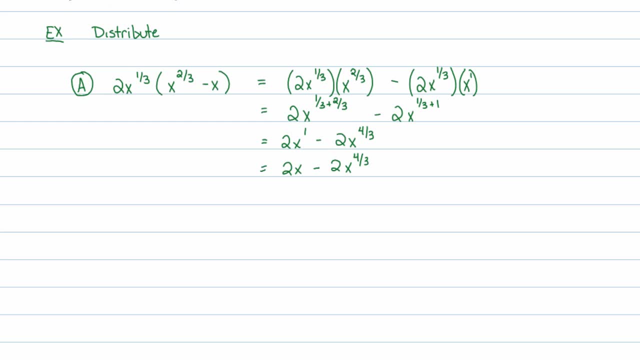 some of this, these markings. Originally I had an object- this one right here- times another object, that one right there, So really I only had one term there. Distribution creates more terms in general, So now I have one, two terms. Often distribution's not a wonderful thing to do. Usually we like to. 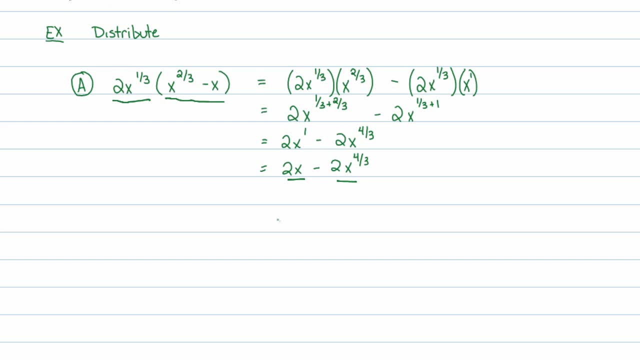 factor because it creates fewer operations. But it's still good to get this practice in. on distribution, And the reason why I think most authors write in distribution first is so you can get used to the idea of distributing And once you start factoring it's pretty easy to realize. 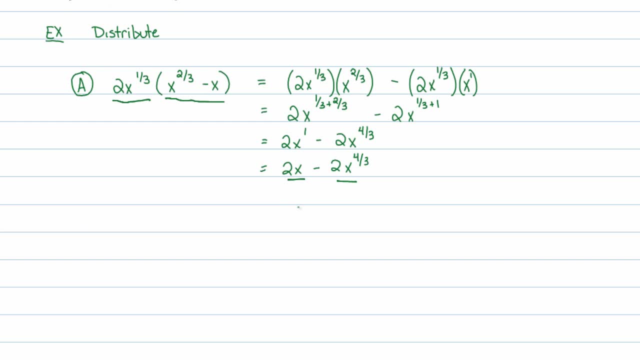 oh, factoring is just the opposite of distributing, So it's the anti-factoring or the anti-distribution, sorry. So let's take a look at this next example: One-third z to the negative, one-half times the quantity z to the three-halves, plus two z to the negative, one-half Again. I'm just being asked to. 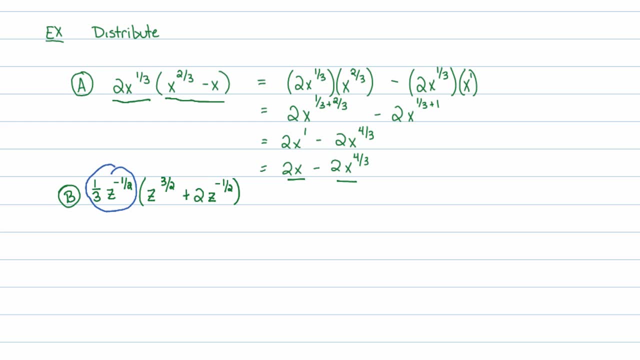 distribute this, so I will. I'll take this monomial out front. It's not really a monomial, I really shouldn't say that. I'll take that expression out front and I'll distribute it to each of the terms. And I'll distribute it to each of the terms And I'll distribute it to each of the. 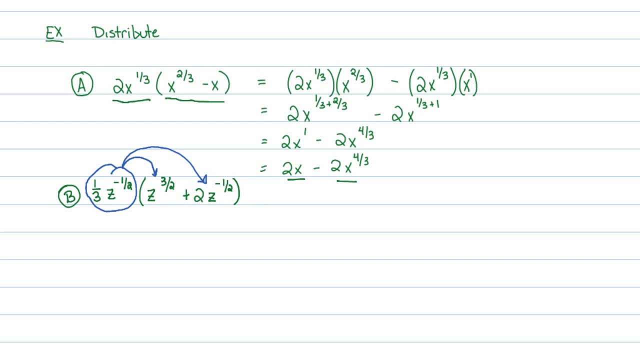 terms here, And so when I do that I'll write out the multiplication kind of slowly. I have one-third z to the negative, one-half times z to the three-halves- It's a little messy the way I'm writing this, Sorry about that- Plus, again one-third z to the negative, one-half times two. 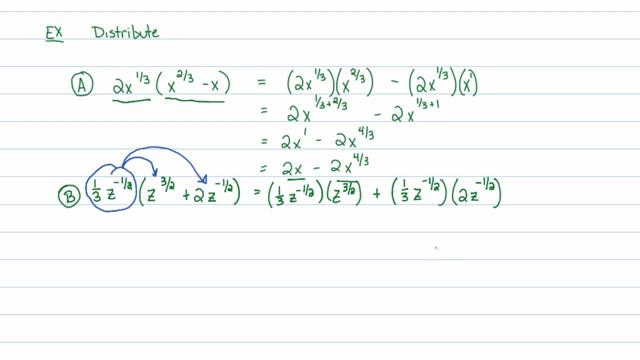 z to the negative one-half. All right, let's clean this up In this first term. here I have one-third and that's it, So just one-third. I'm not multiplying it by any numbers. And I have z to the negative one-half times z to 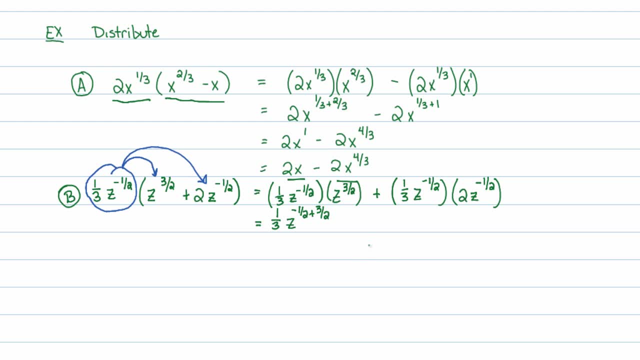 the three-halves, So I'll add their exponents Plus one-third times two is two-thirds Z to the negative one-half, plus another negative one-half. Right, You add their powers. Let's clean this up. That's one-third z to the- let's see negative one-half. 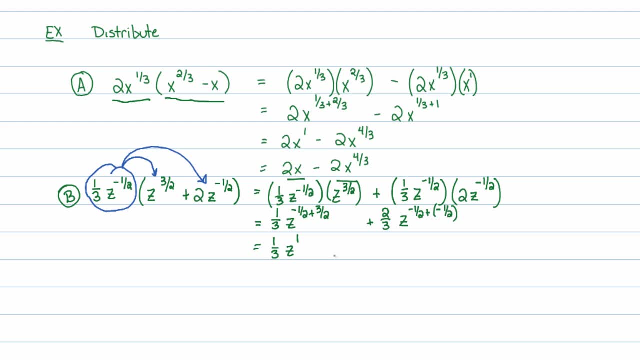 plus three-halves is two-halves, So that'll be z to the first Plus two-thirds Z to the negative. one-half plus another negative one-half is a negative one. Let me just write this one last time a little cleaner: One-third z plus two-thirds Z to the negative one-half. 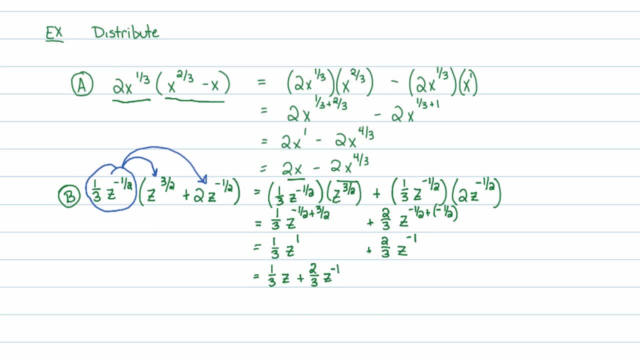 And if you have an instructor that prefers your answers to be with positive exponents, only then you can write this as one-third times z plus two over three z. Right, Because you can rip the negative off that exponent and drop that z downstairs. Now we're going to try the opposite. 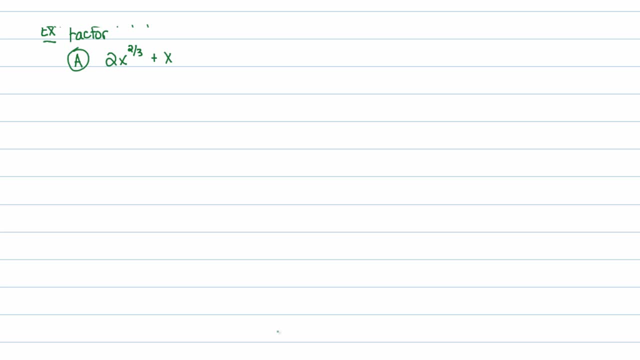 of distribution, which is basically factoring. Well, it's not. basically, It is factoring, But I need to create a new one. So I'm going to create a new one. I'm going to create a new one And I'm going to kind of convince you again, and I've done this in a previous video, but I think it's very. 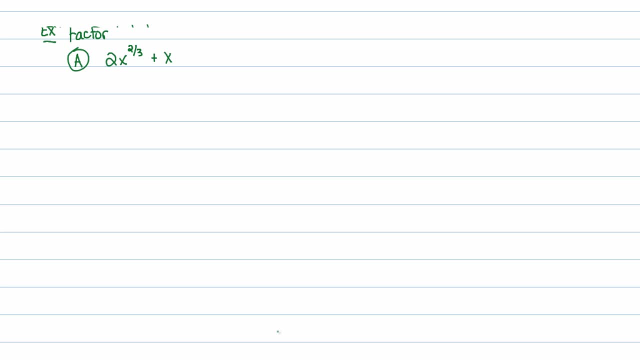 important to see it again that really all you're doing in factoring is that you're pulling out the most negative powered version of, or the least powered version of your variable. For example, if I told you to factor this, well, this is old school, You can easily factor this And you ask yourself: what do? 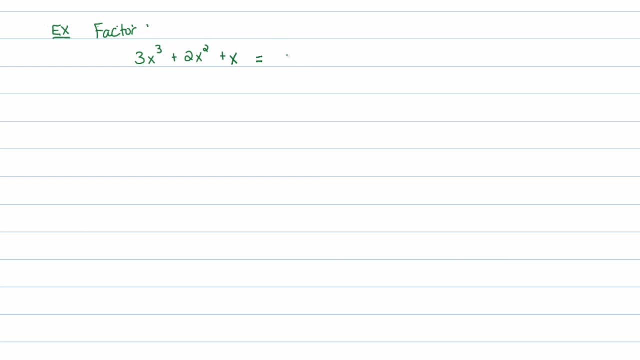 these all have in common And most people would say, oh, they have an x in common. You never really think about why they have an x in common. You never really think about why they have an x in common. You never really think about why you pull out the x. The reason why you factor out the x here is because, well, if you 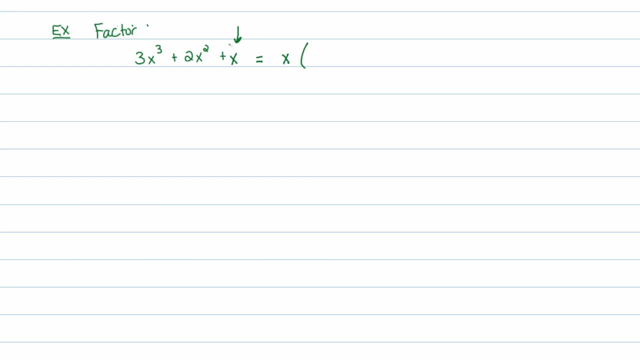 factor out x squared, this third term doesn't have enough power to be able to factor an x squared out of it. If I factor out an x cubed, on the other hand, well, the second and the third terms don't have enough power to. 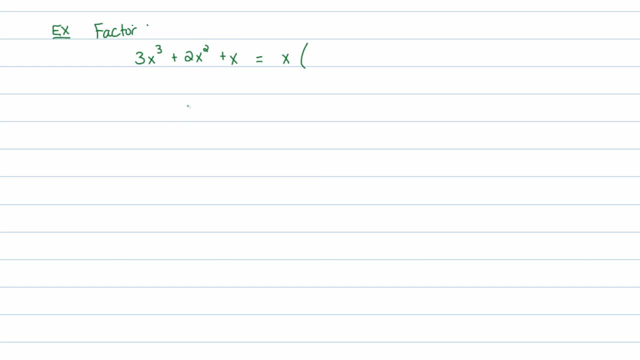 factor out an x cubed. So, that being said, I can factor out an x. Now, just to remind you what factoring is, it's dividing out a variable. So, in other words- and normally you wouldn't have to do this- You do this kind of automatically in your 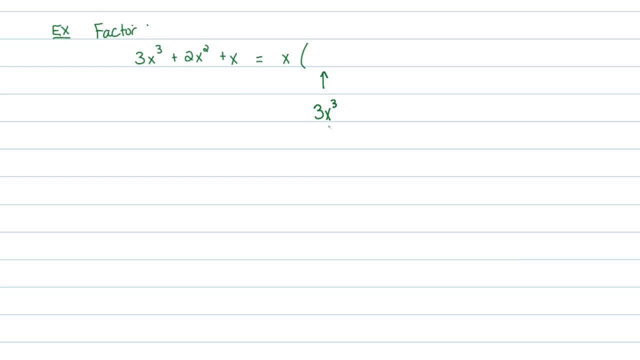 brain. What we had there was a 3x cubed, and we're dividing off a power of x, So in reality, that would be a 3x. oops, I wrote a 2. It's a 3x squared, So that's what we'll go there: 3x squared Plus. well, what was in this place was a 2x squared. 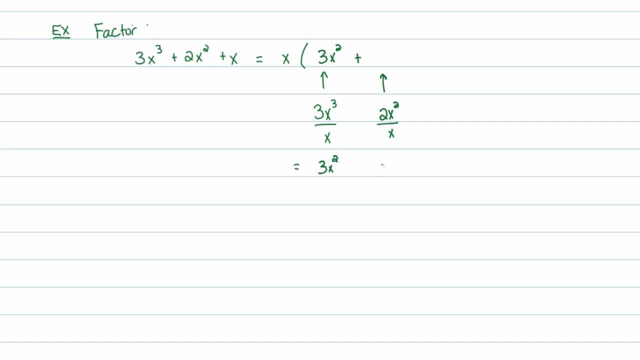 But we're dividing off or factoring out an x, And so that's going to equal just a 2x. And finally, let's see plus. in this last spot we had an x and we're factoring- oops, we're factoring off an x. Let me just keep everything the same. There we go. Factoring off an x is the same thing as dividing out an x. Well, x over x is equal to 1.. So this is plus 1.. 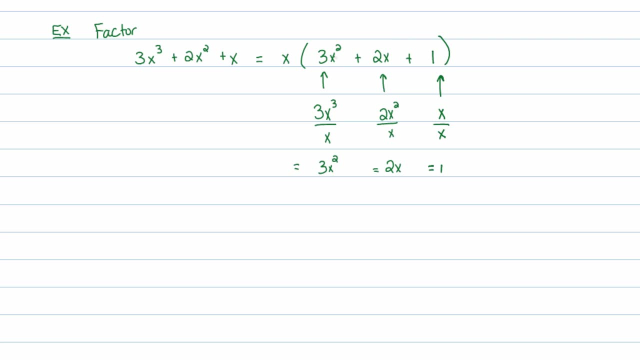 By the way, when you reach the end of this, you should always ask yourself: is this the final answer or can I factor this further? Well, you could try to factor 3x squared plus 2x plus 1, but you may find that it doesn't factor Because you need a 3x and an x and a 1 and a 1 plus and a plus, And if you did this- oh, that was supposed to be a plus. When you did this- you'll find out you get 3x squared plus 4x plus 1.. So this actually does not factor. 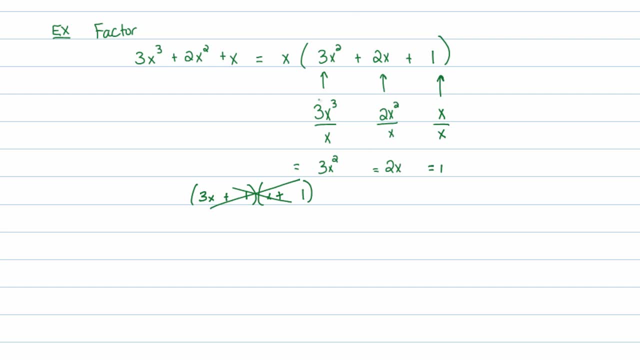 But that's how we normally factor polynomials. Well, the idea of factoring polynomials and factoring expressions is pretty much the same. You factor out common factors or, better yet, rule of thumb, and maybe I'll create a new page for this- When asked to factor, always pull out the lowest powered version of a variable. Now, I was going to say pull out the lowest powered version of all common variables. But I'm going to say pull out the lowest powered version of all common variables. 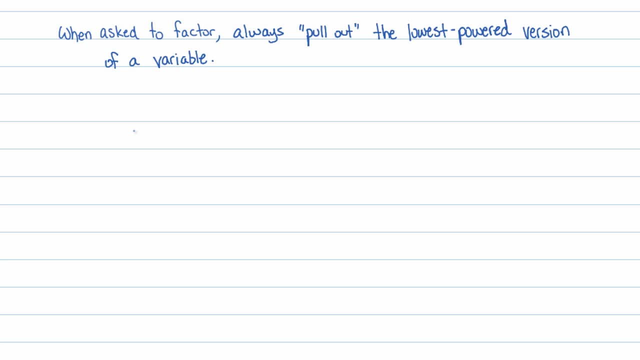 The fact is, sometimes you will pull out a lowest powered version of a variable, even if one of the terms doesn't have that variable. So maybe I'll have an example like that in this example set, But for now, the example that we're being asked to factor here. both of the terms have x's, So let's take a look at this. The lowest powered version of x here will be the 2 thirds powered right, Because the other one has a power of 1.. So what's smaller, 2 thirds or 1?? Well, 2 thirds is. 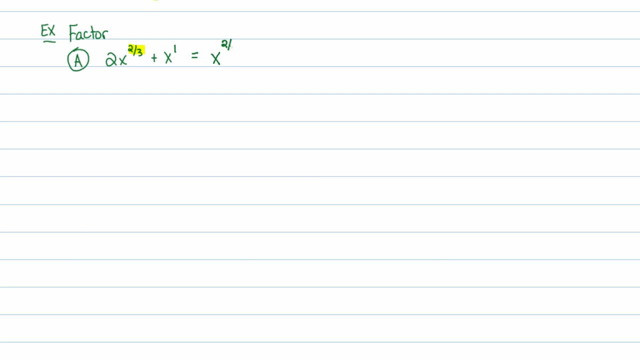 So what I'm going to do is I'll factor out x to the 2 thirds And I'll be left with something in its stead. Well, let's see In that first place we had 2x to the 2 thirds. But we're factoring out x to the 2 thirds And it's pretty easy to see that those x to the 2 thirds will cancel. They're the same picture And they'll just become 2.. So this will be 2, right there. 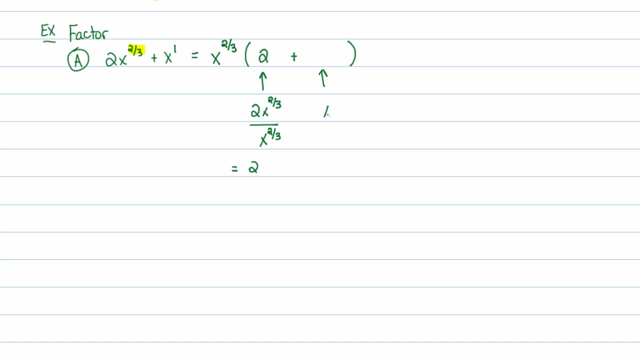 Plus. well, in this spot the term was x to the 1st And we are factoring out x to the 2 thirds. Well, let me just convince you here: x to the 1st is the same thing as saying x to the 3 thirds. So if I have x to the 3 thirds on top, x to the 2 thirds on the bottom, who wins, and by how much? The top wins? It has more power by 1 third, So that's x to the 1 third. 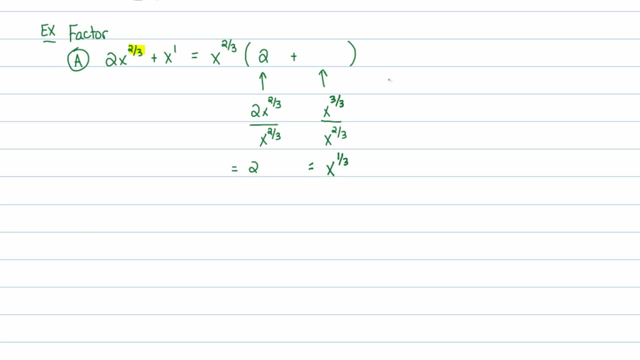 Now I use that language- who wins and by how much? But your instructor might say: listen, just do the law, one of the laws of exponents, which is take the top exponent and subtract off the bottom exponent. That's fine too. You get the same answer. 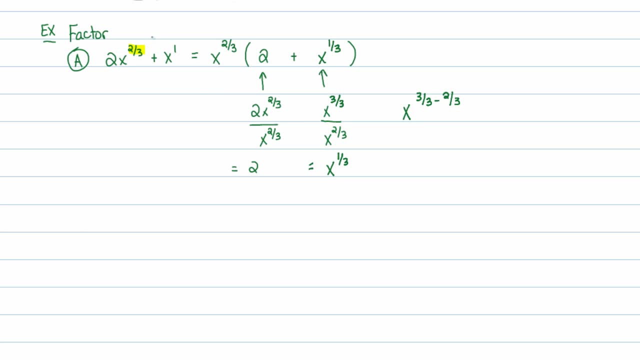 But here we have it. So this is the factored version of 2x to the 2 thirds plus x. It is going to be x to the 2 thirds times the quantity 2 plus x to the 1 third. Now, honestly, this factorization is kind of trivial. There's not a lot that we gain by doing this. 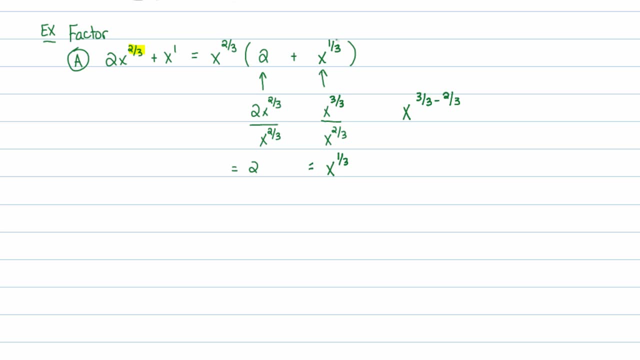 But it is an introduction to factoring. Honestly, the gains that we get in the long run for factoring far outweigh the trouble that we go through. It's just that in this problem specifically, we don't get any computational gains, But look at what we have here. This is exactly what it's telling you when I wrote down. let me pop down a couple. 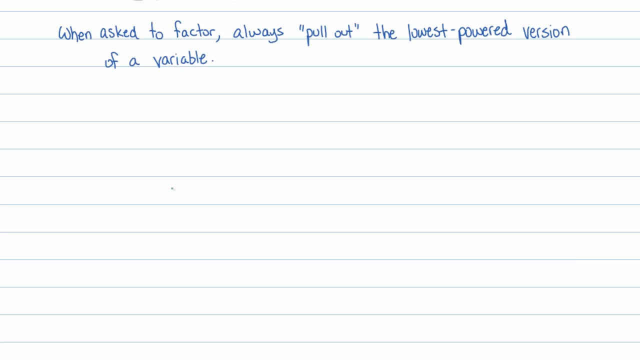 when I said, when asked to factor, always pull out the lowest powered version of a variable instead of the common variable. Notice that each term- here all three terms- do not share a variable in common, So a lot of people would think you can't factor anything out of this. 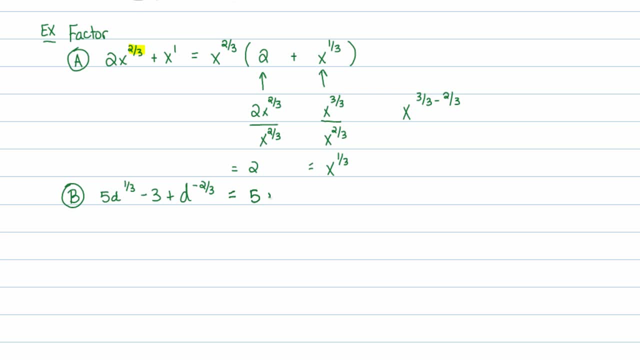 But in reality I could write this to where they share a variable in common. This is 5d to the 1 third, minus 3d to the 0th, plus d to the negative 2 thirds. Often I'll get students that ask me: well, am I supposed to do this from now on? 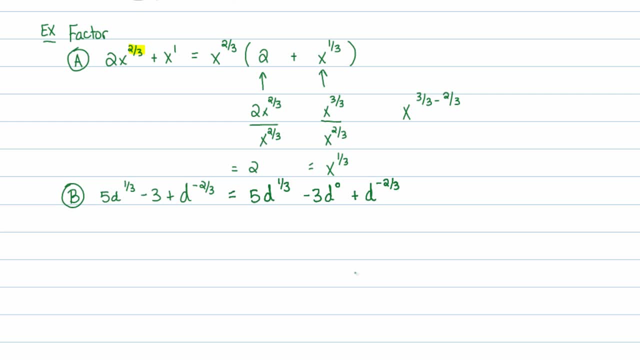 Am I supposed to? Am I supposed to do this from now on? Am I supposed to actually, you know, write d to the 0th whenever I have a constant, Or, yeah, a constant term? The answer is really no. 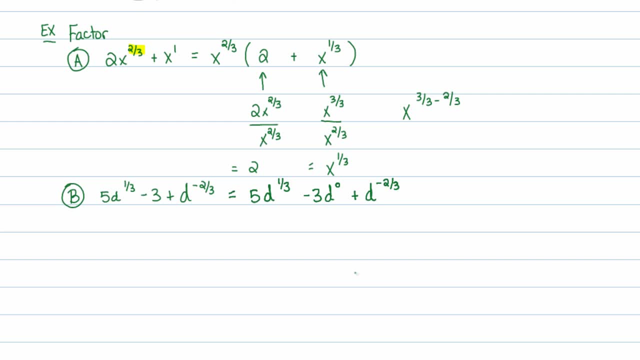 This tactic is only really useful if you have negative exponents. Yeah, really only useful if you have negative exponents. That's really the only time you need to consider doing something like this. So if you do have an expression like this and you're asked to factor, 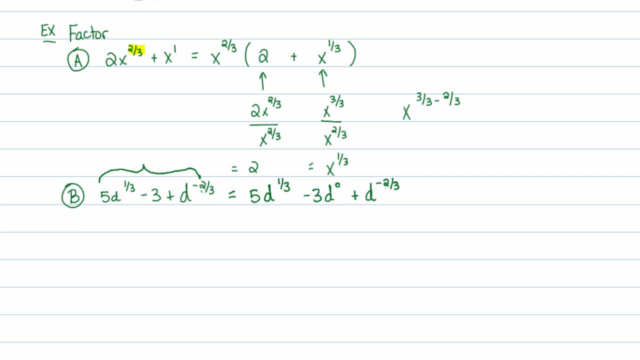 and you notice that one of your exponents on your variables is negative, then likely, you can factor as long as you put a variable to the 0th power on the constant. Now, when I look through each of these three terms that all have d in common now, 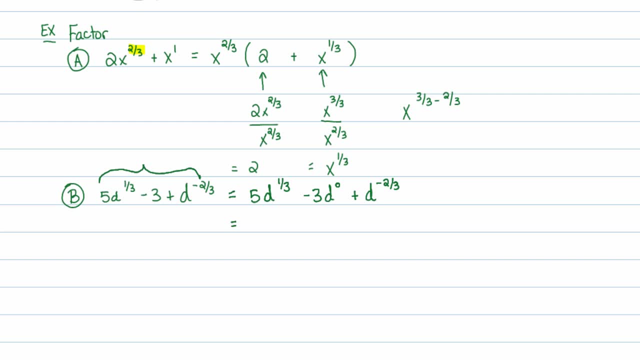 I'm going to factor out the lowest powered version of that d and that would be the negative 2 thirds. That's the lowest, the most to the left on the number line. So if I pull that out front I'll have d to the negative 2 thirds out front. 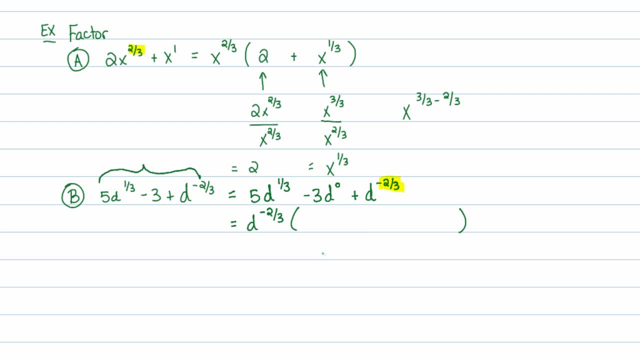 and I'm looking at the number line, and I'm looking at the number line and I'm left with some junk on the inside. Well, let's figure out what that junk is. In this first term slot, we had 5d to the 1 third. 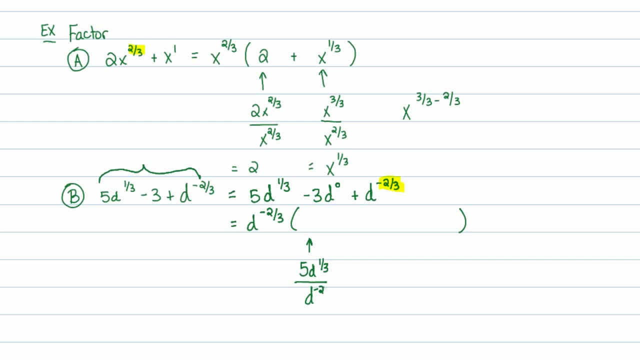 but I'm factoring out d to the negative 2 thirds. Now, remember, I can rip that negative off that exponent and pop that d to the 2 thirds upstairs. So that's what I'll do. I'll write this as 5d to the 1 third times d to the 2 thirds. 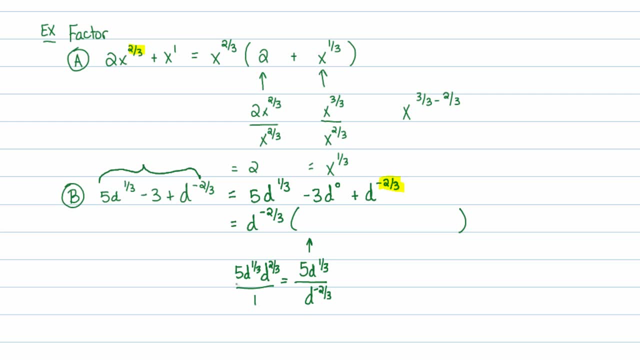 because I ripped off the negative. it hops upstairs And now I see that I have d to the 1 third times d to the 2 thirds, so I can actually multiply those two. It's 5d to the 1 third plus 2 thirds, which is just 1.. 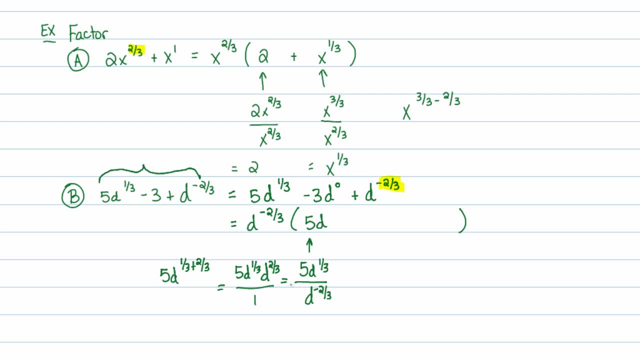 So this is going to be 5d right here to the first power, The next one minus. I had 3d to the 0th, or basically 3.. And I'm dividing that by 2.. So I'm dividing out d to the negative 2 thirds. 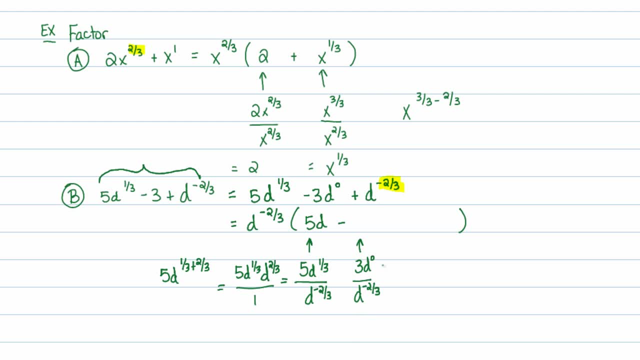 Again, rip the negative off that exponent and pop d to the 2 thirds upstairs. So this will become 3d to the 0th plus 2 thirds, or in other words 3d to the 2 thirds. Finally, plus. 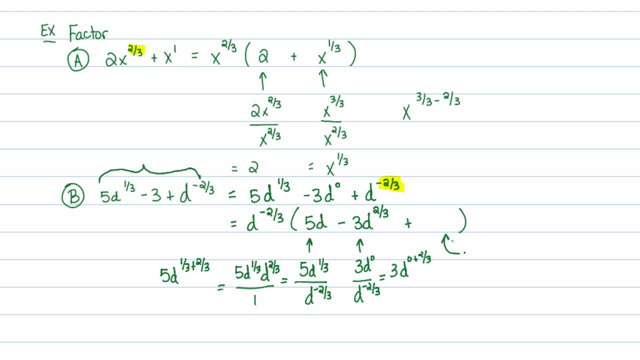 We had d in this spot, right here. We had d. We had d to the negative 2 thirds, But I'm factoring out d to the negative 2 thirds. Well, you can easily see those are going to cancel and become 1.. 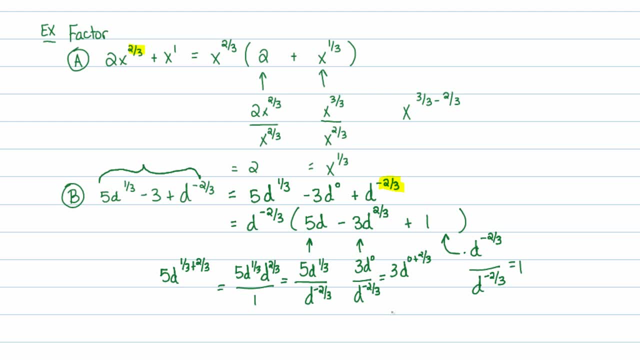 So this is just plus 1.. There you have it. That's not so bad. I mean, we factored all that out. We do get some annoying exponents here, But still not so bad. Now, I didn't mention in the last example. 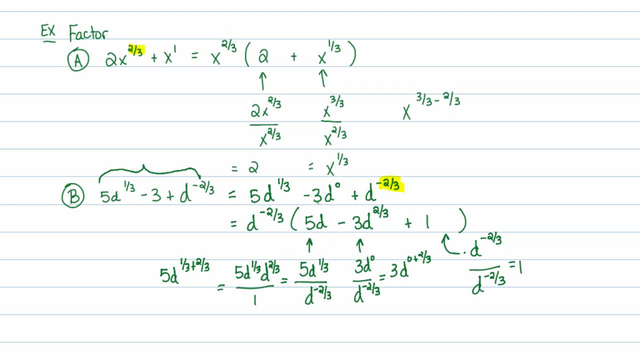 but you should check to see if you have any exponents here. You should check to see if this factors any further Now, because this is not really a quadratic in here, but we have three terms. it really doesn't factor, So I'm just going to move on from this one and go into the next example. 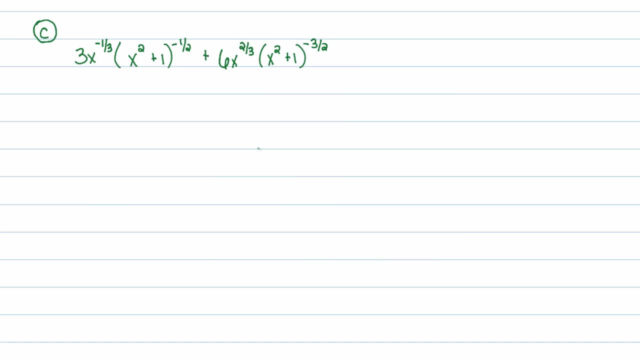 Now here comes the beast. This is the one that is going to take a little bit of thinking to factor. But just remember, when you're factoring, you're considering first of all how many terms there are. And I look at this. 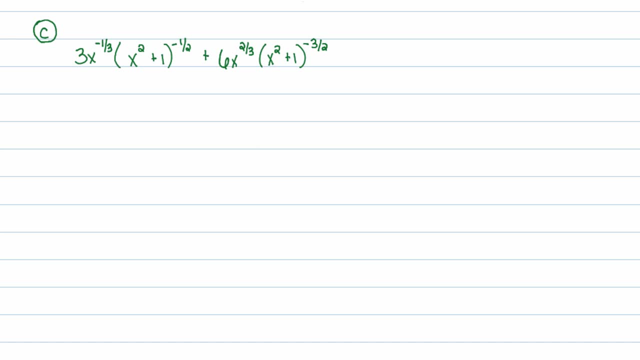 I see there's a term right here. I'll just highlight it really quickly. Here's a term and here's the second term, So we have two terms. Each of those terms might have things in common. They might not. If I take a look at them, though, I know that they both can be divided by 3.. 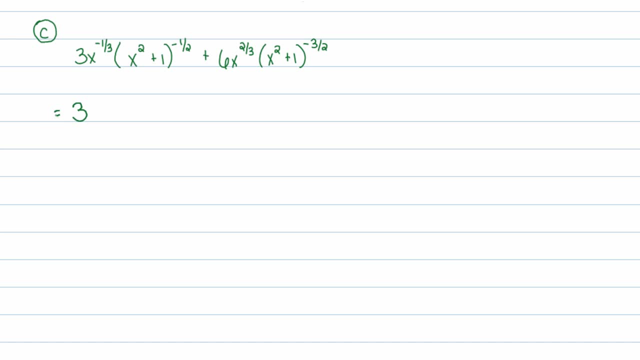 So I'll pull a 3 out front. They both share x, So I'm going to write x. And remember you're looking for the lowest powered version of that x, which would be the negative 1 third right here. So I'm going to. 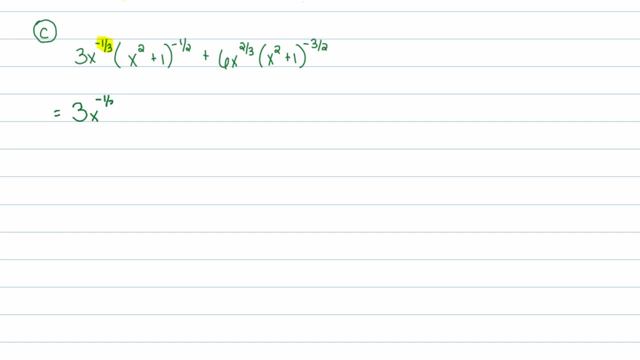 Pull off x to the negative 1 third, And then I'm looking again because I see that they both share. Now this is where you have to use your little, the skills of kind of pattern recognition- I guess you could say- where you kind of step back from the problem. 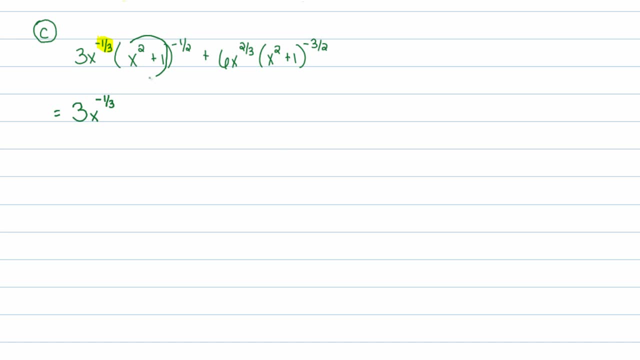 And notice that this picture, this picture right here, is the same as this picture right there, And x squared plus 1 is the same as x squared plus 1.. So you have to pay attention to that And you say, oh, I notice that both of those have an x squared plus 1 in common. 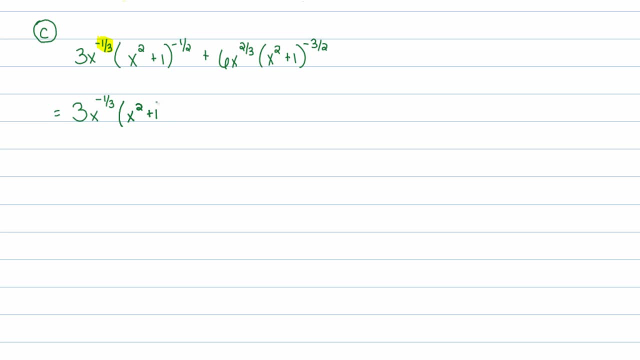 So let me write x squared plus 1.. And again you want to factor out the lowest powered version of that, which is right here. It's negative 3 halves. That's lower than negative 1 half. So I'll write negative 3 halves, right here. 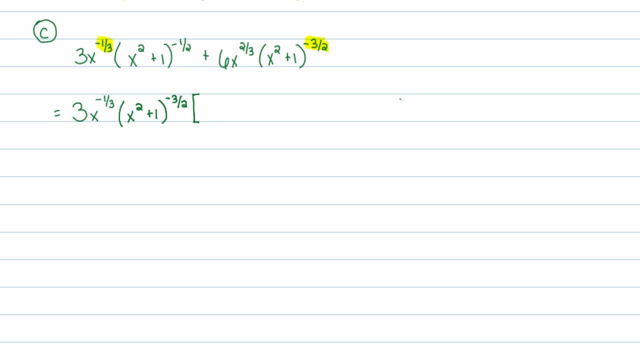 And now you're going to be left with something And I'll write this in braces, like this little brackets. I guess you could say: And here's where it's really important to do that whole business, where I say what was here and I divide stuff out. 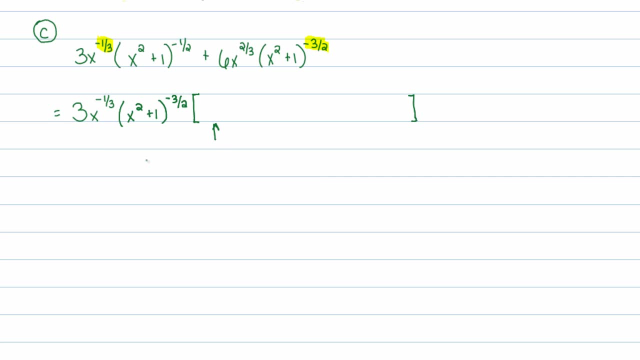 It's very important that you do this. So what was there was a 3x to the negative 1, third times x squared plus 1 raised to the negative 1 half. But what I'm doing is I'm dividing out, pulling out front, basically. 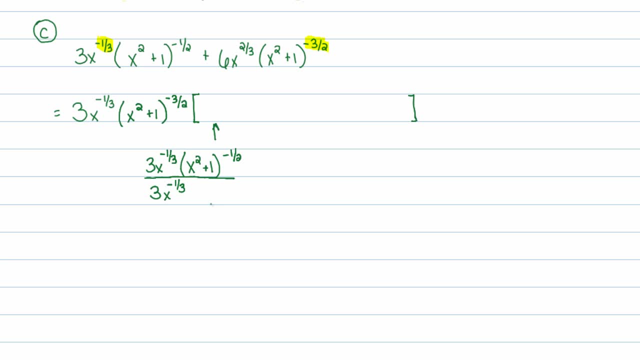 3x to the negative, 1 third times x squared plus 1 raised to the negative, 3 halves. First things first, we can notice that the 3s will cancel nicely. 3 over 3 is just 1.. And in fact, x to the negative- 1 third over x to the negative- 1 third will also turn into 1.. 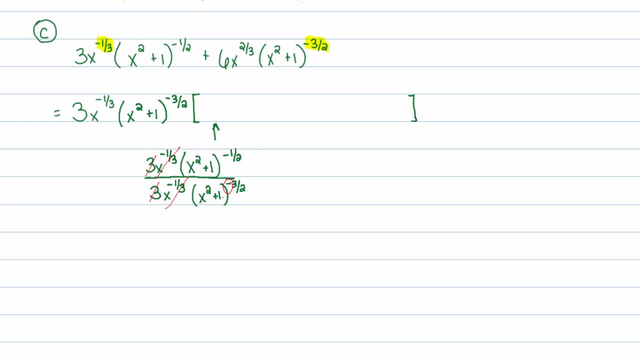 So now I'm going to go ahead and rip the negative off this exponent in the denominator and pop that business upstairs. So this is just going to equal x squared plus 1. to the negative: 1 half times x squared plus 1.. To the positive: 3 halves. 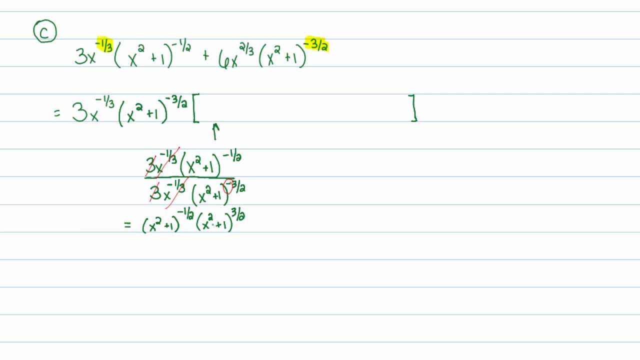 Notice, I didn't really knock that other one downstairs because they're the same base. I'm just going to add their exponents- I'll make them x squared plus 1, to the negative, 1 half plus 3 halves, Or in other words to the first power. 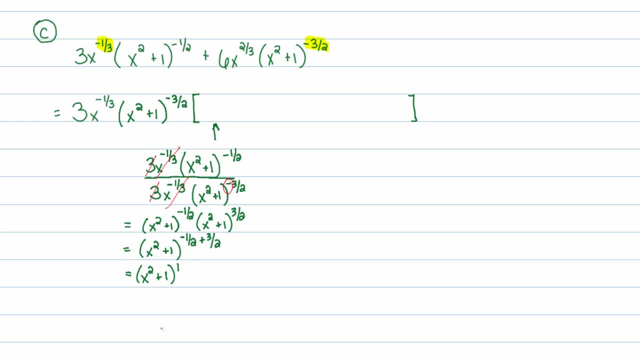 Now that's really not a nice way to write that x squared plus 1 to the first power Same thing as saying x squared plus 1.. So it was a little bit of work getting there, but it's so important for you to write out these divisions like this. 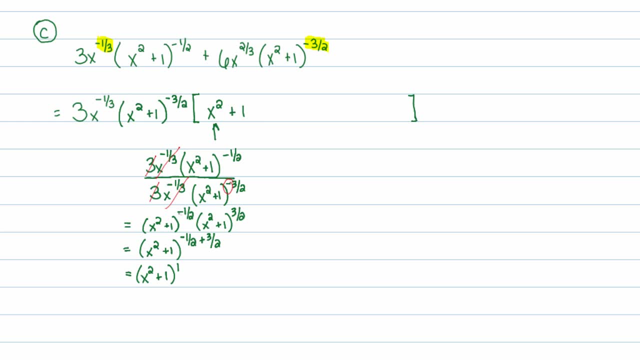 Because that's really what factoring is. It's just dividing out. So it really does help out when you do that, so that you can get down the nitty gritty with the problem and not make too many mistakes. Now I'll write plus here. 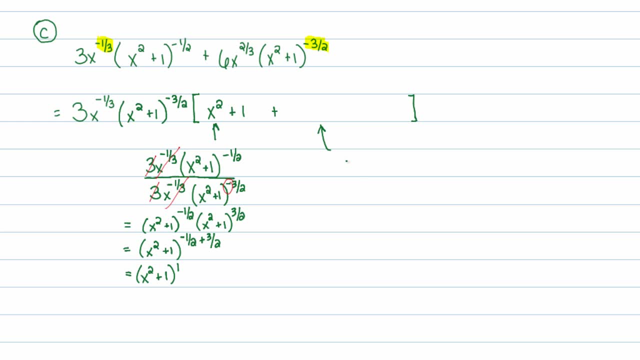 In the second position we had 6x to the 2 thirds times x squared. So that's x squared plus 1 raised to the negative 3 halves, And what we're dividing off of that is 3x to the negative 1 third times x squared, plus 1 raised to the negative 3 halves. 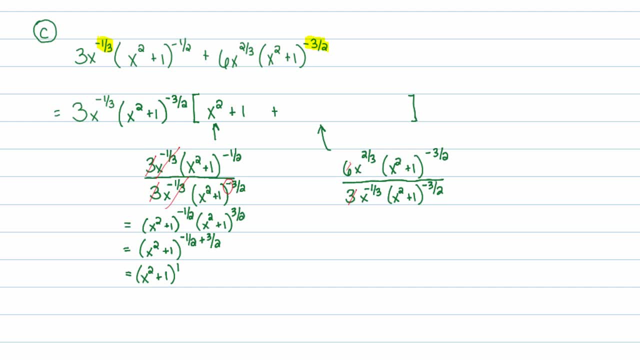 Well, okay, I know that 3 will go into 6 twice And I know that x squared plus 1 to the negative 3 halves is the same thing as x squared plus 1.. So those two cancel out. So this I'm going to rewrite just because it's a little bit messy. 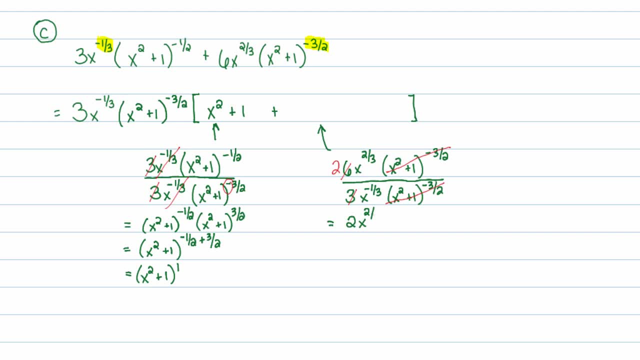 It's 2x to the 2 thirds over x to the negative 1 third. I'm going to rip the negative off that exponent in the denominator and throw that business up top. So that's 2x to the 2 thirds times x to the 1 third. 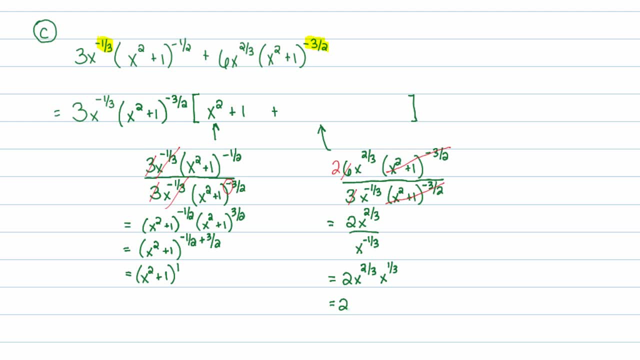 Add the exponents, That will be 2x to the 1, third x to the 1, basically. So right, here will be 2x. Now, something you should note here, And I'm going to erase this now because I don't need to reference it anymore- 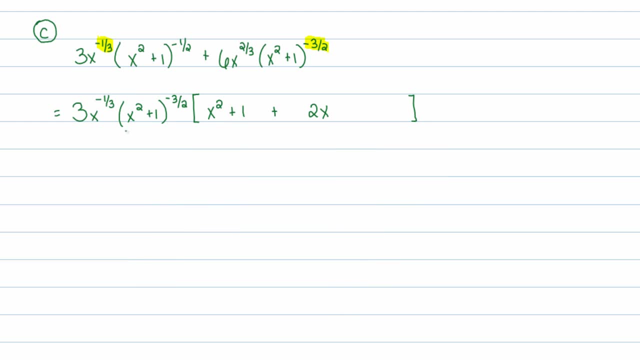 You can always rewind and watch what I did. This can be rewritten, So let me clean this up: 3x to the negative, 1. third times the quantity x squared plus 1 to the negative, 3 halves, And I'll reduce these regular old parentheses. 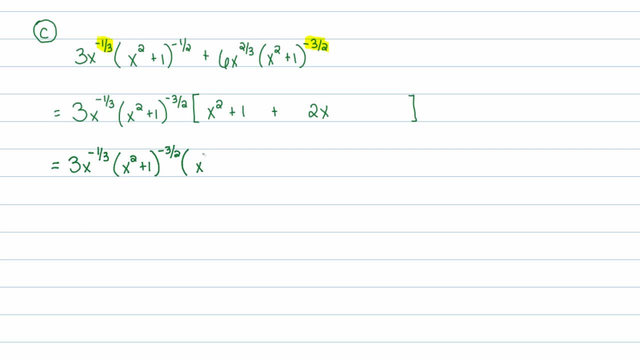 And I'm going to write this in decreasing power order. So x squared plus 2x plus 1.. Last thing you should do here is, after you're done doing a major factorization, which is what we did here. You should breathe a heavy sigh of relief. first of all, 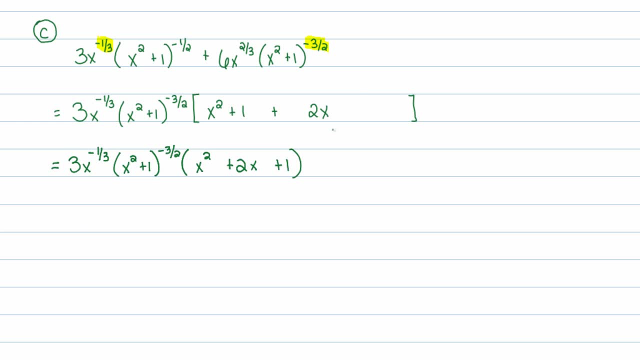 And then, secondly, you should see if this trinomial factors It actually does. It factors to x plus 1 times x plus 1.. So that's going to be 3 times x. Well, you don't want to hear me say this out loud. 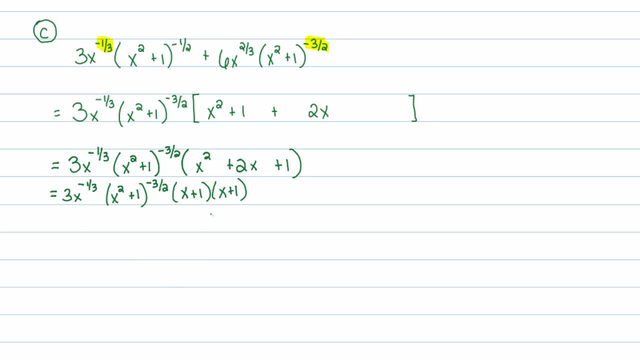 I'll just rewrite it Now. leaving it like this is pure laziness. So you should combine these two to be an x plus 1 quantity squared Voila, we are done. If your instructor requires you to leave your answers with positive exponents only. 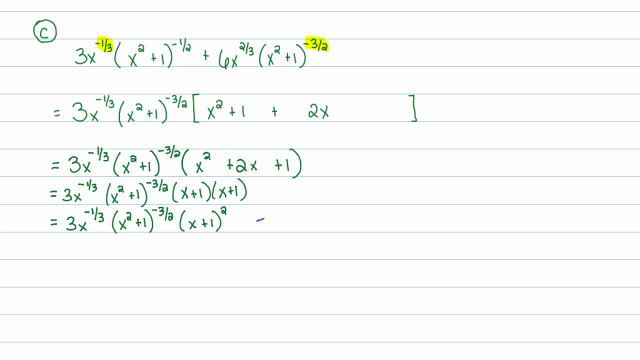 well then go ahead and pop this stuff downstairs. That's okay with me. That would be 3 times the quantity x. That would be x plus 1 being squared, And everything with negative exponents here will pop downstairs. So you'll have x to the 1 third and quantity x squared plus 1 to the 3 halves. 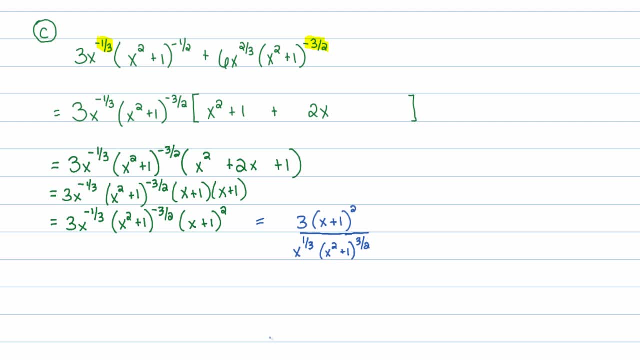 Okay, that's pretty much all I need to say about factoring and distribution with rational exponents. I mean, that's all the advanced factoring there is. Everything else from this point forward is just repetition. So you just need to be very aware. 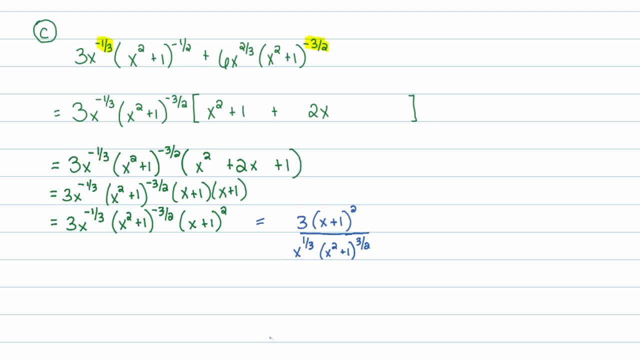 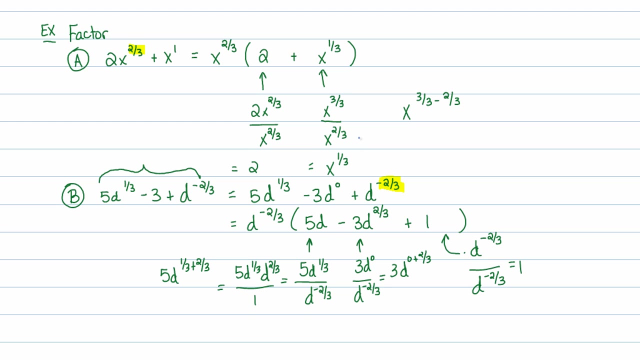 Always pull out the lowest power version of your exponent or of your variable And then do a slow division, like I have been doing in each of these problems. So, for example, all this stuff right here. Just make sure you do slow divisions like this so that you keep track of all your steps. Okay, Thank you, Bye, Bye, Bye. 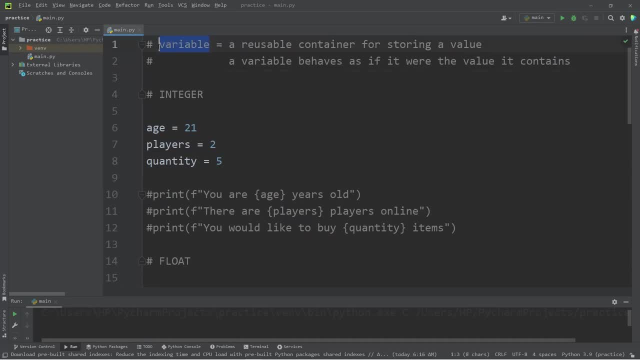 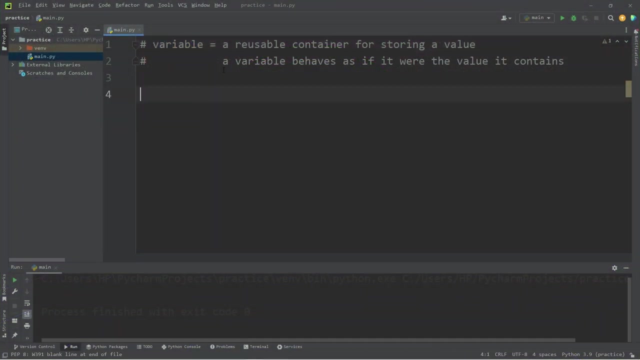 Hey, what's going on everybody? In this topic? I'm going to explain variables and data types in Python, as well as give you a few useful tips and tricks at the end of this topic. So why don't you sit back, relax and enjoy the show? Let's talk about variables. A variable is a reusable. 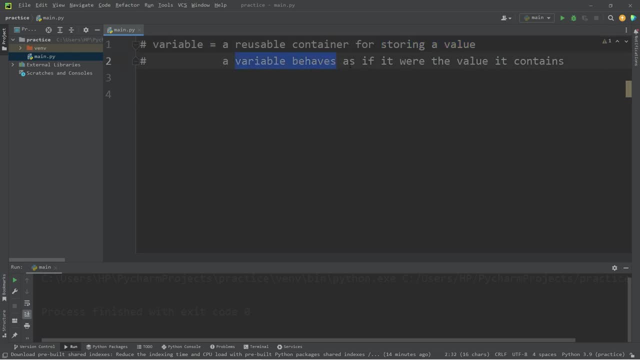 container for storing a value, A variable behaves as if it were the value it contains. Think back to algebra class back in the day. We have an equation that contains x. X is some representation of a value. Wherever we use x, it behaves as if it were a certain number. That's kind of the same. 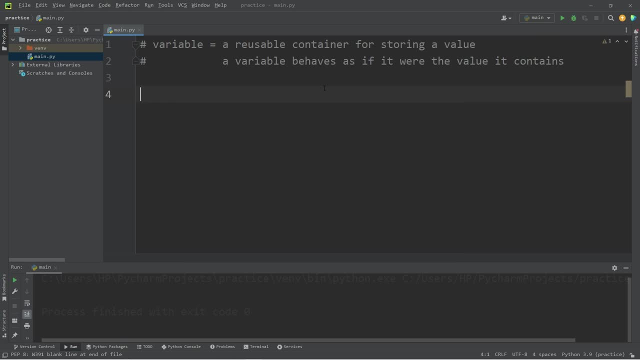 thing with programming. Now, when we create a variable, we would like to give a descriptive and unique name of what that variable contains. Suppose I'm working with a user's age, I could declare a variable named age. Age equals then some value. Let's say, my age is 21. Not anymore.